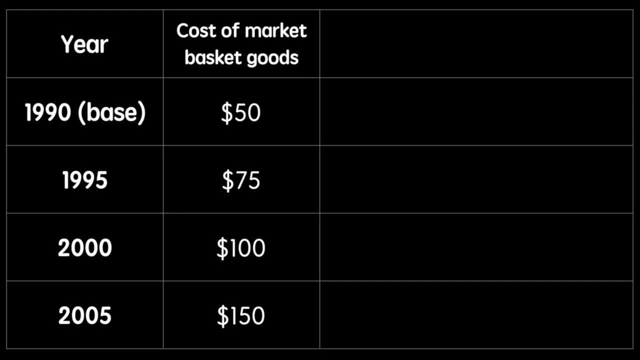 pricing prices and we'll use this information in the final column to calculate our price index. The CPI is calculated by dividing the current price of the market basket by the market basket of the base year, which is then multiplied by 100.. It's also very important. 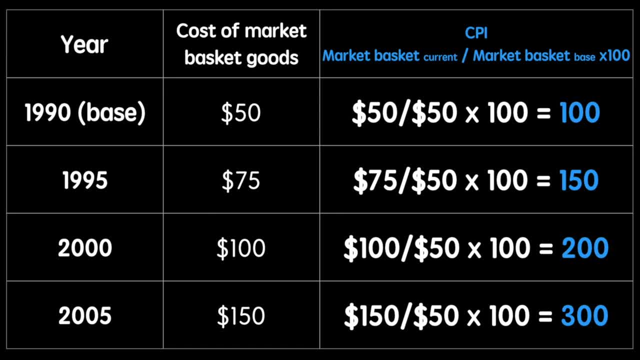 to remember that the CPI is not a percentage, so we don't add a percent sign afterwards. Applying this formula to each year, we are able to arrive at the consumer price index from 1990 to 2005.. I've used simple calculations to illustrate, but you may see some examples. 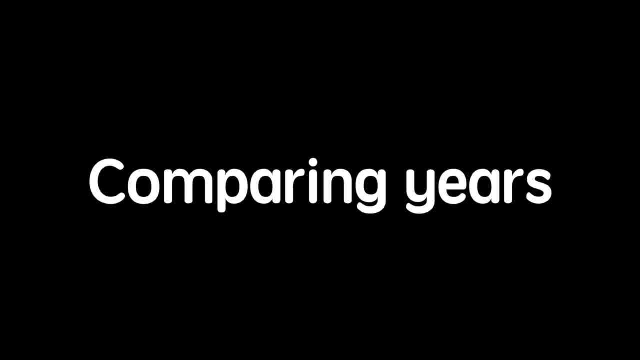 that are slightly more complicated than this. By looking at the CPI over years, we can calculate the inflation rate. Let's see how that works. In this table we'll lay out the same years and the CPI we calculated for each year As. 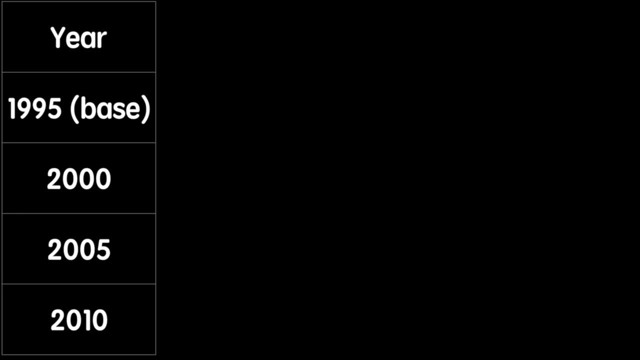 we're always comparing to the base year. we'll also calculate inflation for each year compared to the base year of 1995.. When calculating the inflation rate, it's vital that you subtract the CPI of the comparison year from the CPI of the new year and then divide by the value. 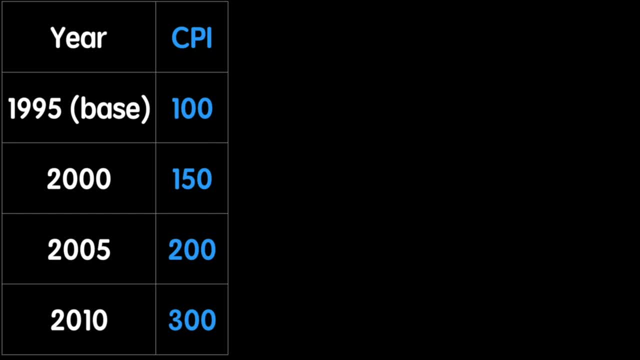 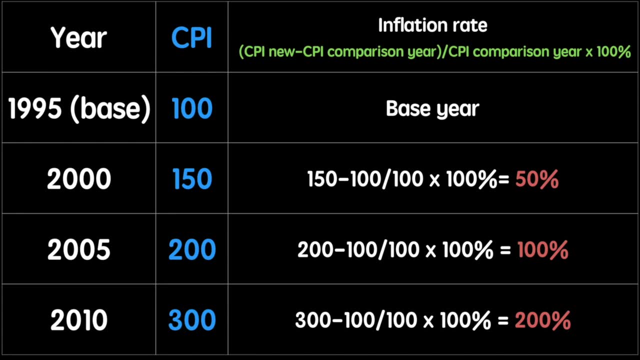 of the comparison year. We don't always calculate inflation against a base year, and it's far more common to see year-on-year comparisons as inflation as well as monthly comparisons. The information provided in this slide is just to act as an illustration. The following: 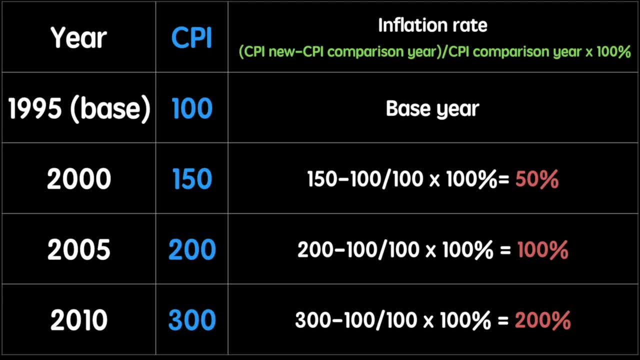 inflation rates have been calculated for each year. We always include the percentage sign when calculating the inflation rate. Always ensure that your calculations are written out as such, if necessary. Don't skip any steps in your work when responding to exam questions. Although these calculations help provide us with a picture of inflation and how prices 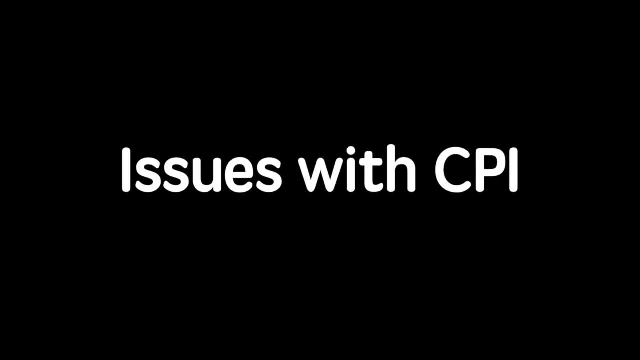 are changing. there are some issues surrounding the use of CPI as a measure of inflation. A typical household does not represent every household. The market basket used in the CPI is based on its purchases made over long periods. It is generally fact жеes in times of great. 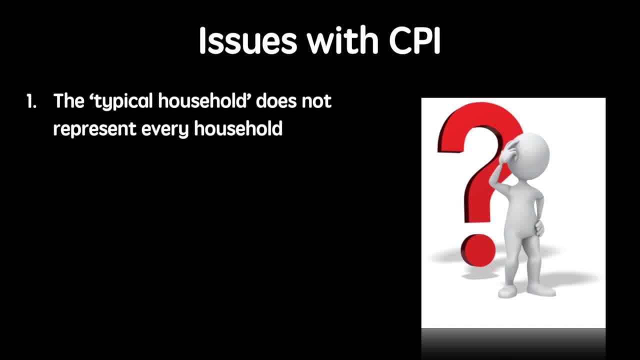 strolls, andemics. A typical household does not represent every household. The market basket used in the CPI is based on purchases made by a typical household. It is not an exact science and since we tend to buy different goods and services, the CPI does not apply equally to us all. 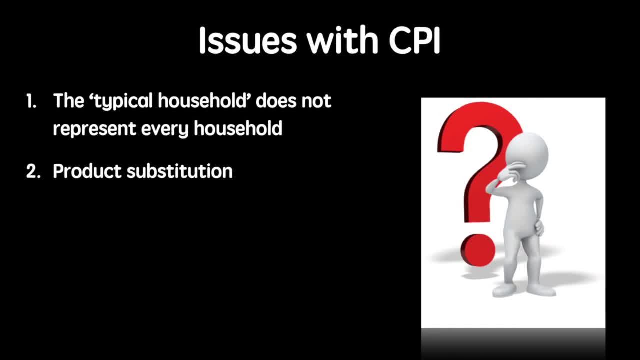 2. Product substitution. As goods and services become more expensive, people switch away from them. For example, if beef becomes more expensive, people may start consuming more lamb. Therefore, the CPI can overstate inflation if it accounts for goods and services that